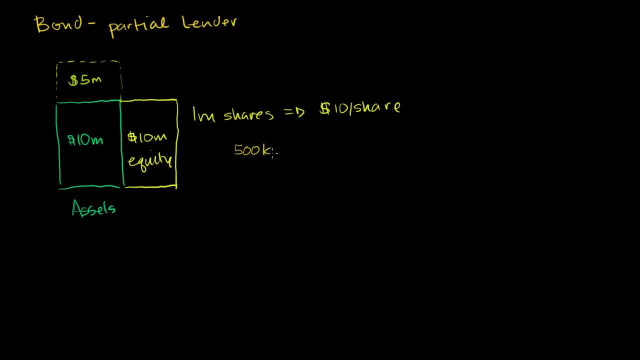 issue another 500,000 shares at $10 per share, And then that would essentially produce $5 million. So this is scenario one: They issue 500,000 shares at $10 a share. They now have 1.5 million shares, but these new owners. 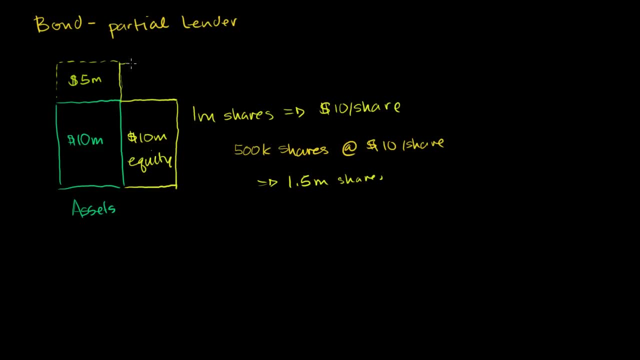 gave them collectively $5 million, So the equity would grow by $5 million. We now have 1.5 million shares, So this would now be 1.5 million shares, not 1 million, And that new money from these new shareholders would go into. 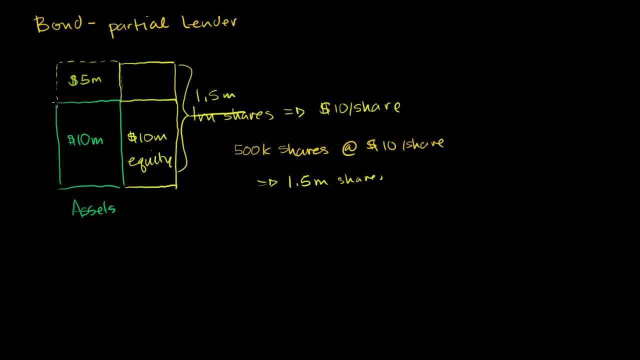 the asset side, and then we would use that to actually buy the factory. What I just described, What I just described, is essentially issuing equity or financing via equity or by issuing stock. Now, the other way to do it is to borrow the money. 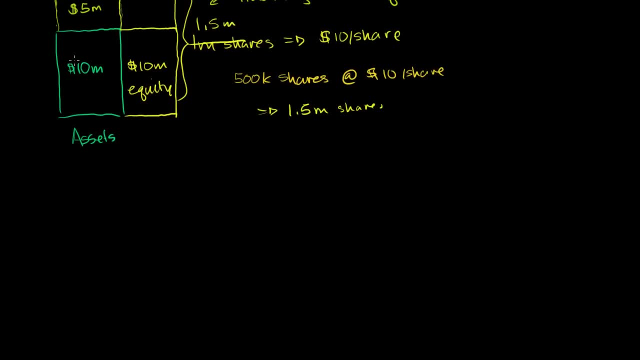 So let me redraw this company. I'll leave this up here just so we can compare the two. So once again, we have $10 million of assets. That's our $10 million of assets. We have $10 million of equity to start off with. 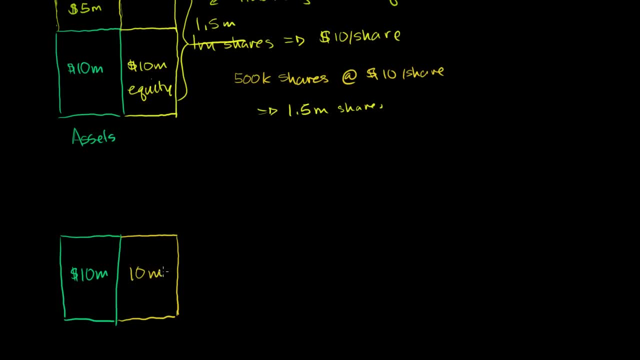 $10 million of equity And instead of issuing stock to get the $5 million, we're going to borrow the money. So we're essentially issuing debt. So we could go to a bank and say: hey bank, can I borrow $5 million? 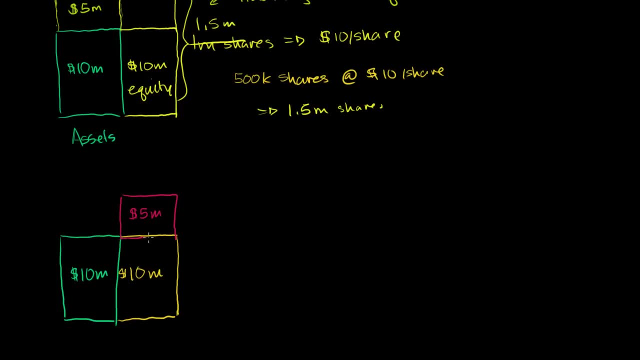 So we would have a $5 million, $5 million In liability- it would be debt, $5 million of debt- And the bank would give us $5 million of cash that we can then go use to buy our factory. So in either situation, the asset side of our balance. 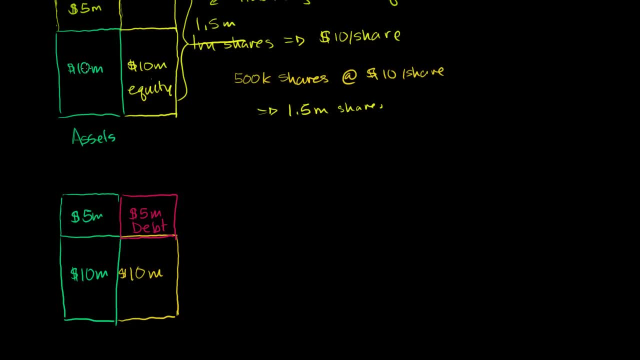 sheet looks identical or the assets of the company are identical. We had our $10 million assets and now we have a factory. But in this first situation I was able to raise that money by increasing the number of shareholders, by increasing the number of people that I have to split the 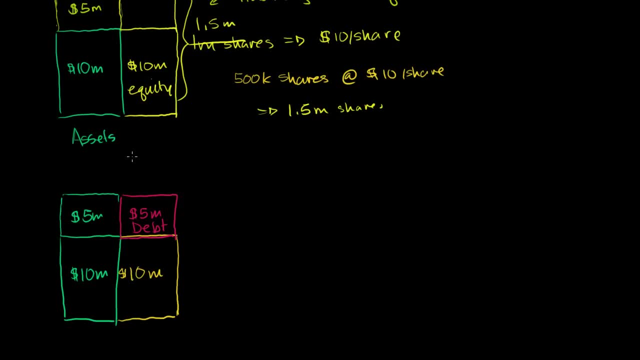 profits of this company with. In this situation, I was able to raise the money by borrowing it. So the people that I'm borrowing this money from this is borrowed money. They don't get a cut of the profits of this company. What they do is they get paid interest on their money. that 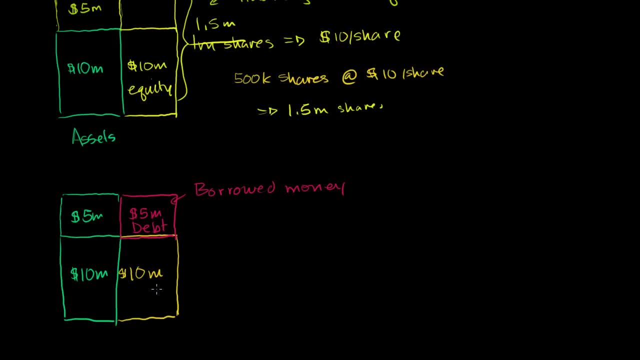 they're lending to us before. these guys get any profits at all. In fact, that interest is considered an expense. These guys get interest and even if this company does super, super well and becomes very, very profitable, these guys only get their interest. 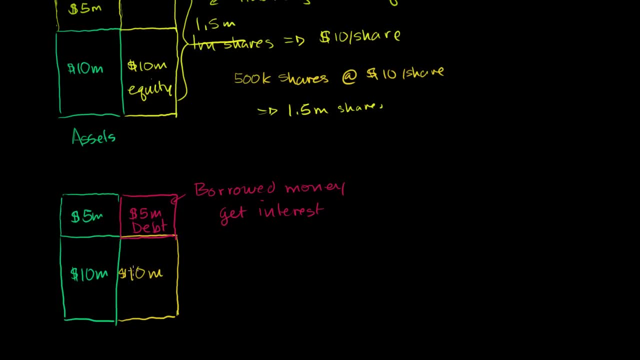 Likewise, if the company does really bad and these guys suffer, as long as the company doesn't go bankrupt, these guys are still going to get their interest, So they're going to be a lot safer than well. they don't get as much of the reward as the new equity holders would. 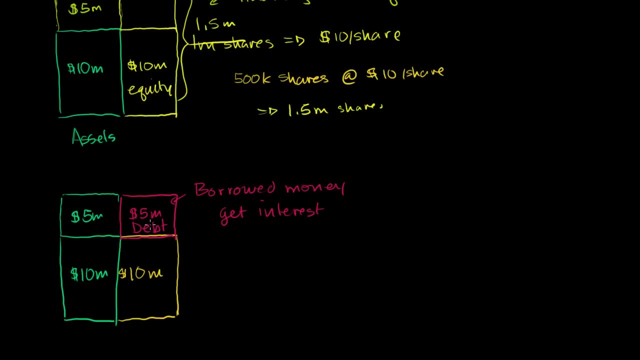 They also don't get as much of the risk. Now, this is just straight up debt And you could just get this from any bank if they were willing to. If they said: oh, you're a good, safe company, We're willing to lend you $5 million. 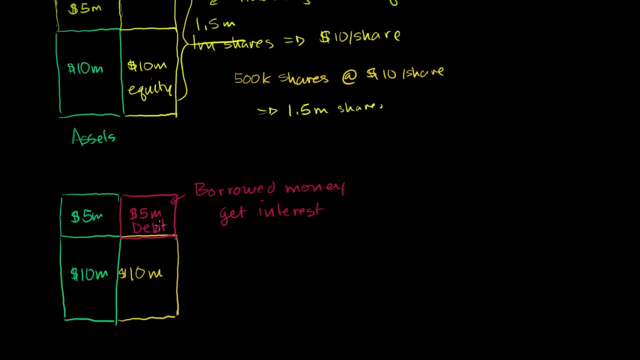 But let's say that no bank wants to individually take on that risk. So you say, hey, instead of borrowing $5 million from one entity, why don't I borrow it from 5,000 entities? So what I can do instead, instead of borrowing it from 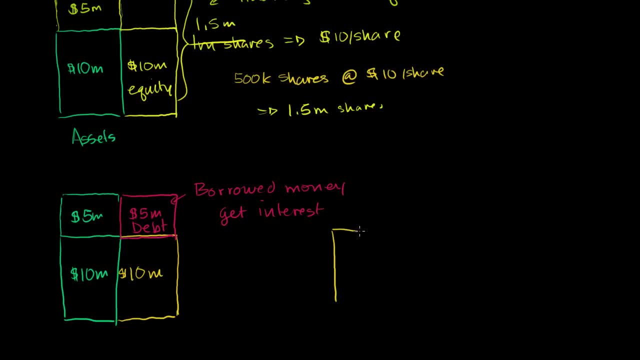 one entity. I could issue these certificates, I could issue bonds, And that's the topic of this video. So I issue these certificates. They have a face value of $1,000.. Or sometimes you'll hear the notion of par value. 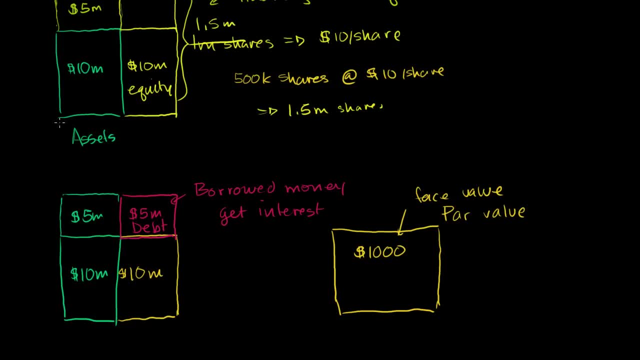 And I'll say what interest I'm going to pay on it. So let's say it has a 10% annual coupon. Even though this is the interest, I'm essentially going to pay $100.. Yes, I'm going to pay $60. 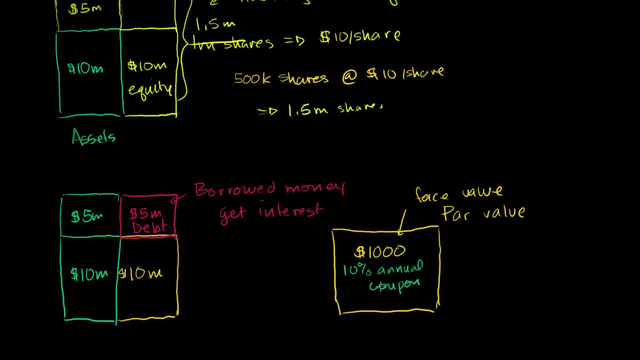 dollars a year. It's called a coupon because when bonds were first issued they would actually throw these little coupons on the bond itself And the owner of the certificate could rip off or cut off one of these coupons and then go to the person borrowing or the entity borrowing the money and get. 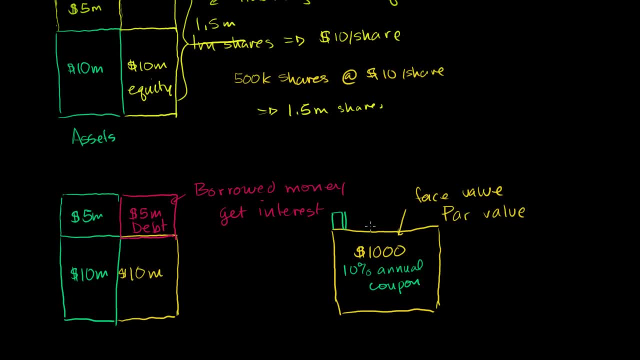 their actual interest payment. So that's why it's actually called coupons, But they don't actually attach those coupons anymore. And then it has some maturity date, The date that not only will I pay your interest back, but I'll pay the entire principal, the entire face value. 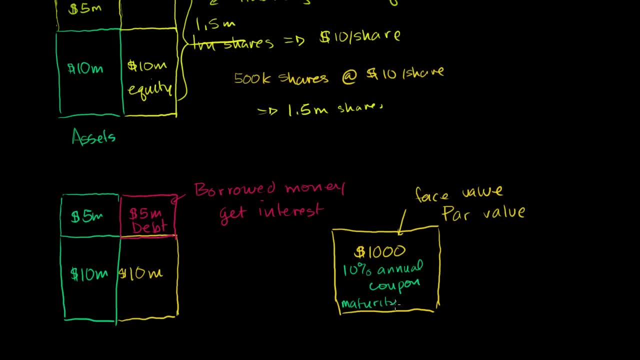 So let's say, the maturity is in two years. So in this situation, in order to raise $5 million, I'm going to have to issue 5,000 of these, Because 5,000 times 1,000 is 5 million. 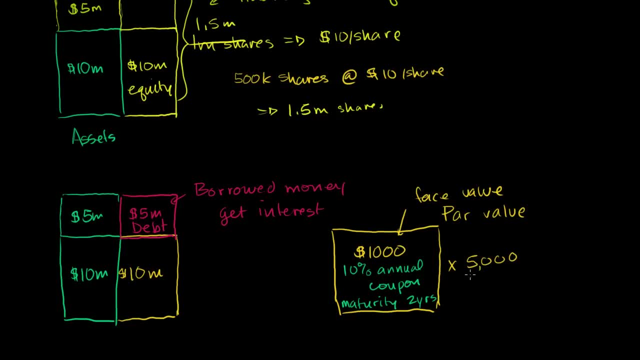 So times 5,000.. So if you wanted to lend $1,000 to this company so that they could expand, and if you think 10% is a good interest rate And it's a safe, It's a safe company. 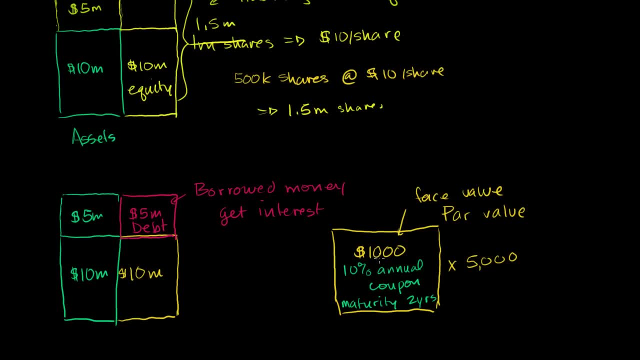 You would essentially buy one of these bonds. Maybe you buy it for $1,000.. And when you buy that bond for $1,000, you are essentially lending this company that $1,000.. And if you did that 5,000 times, or if that happened 5,000. 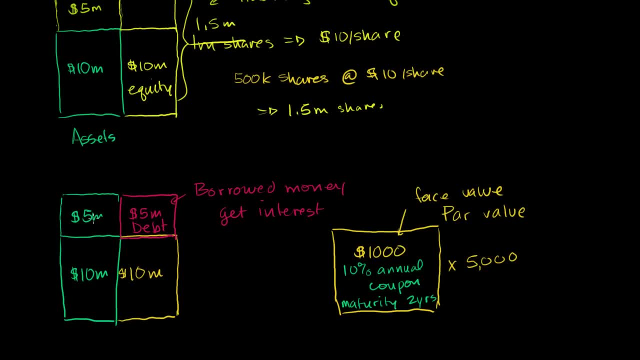 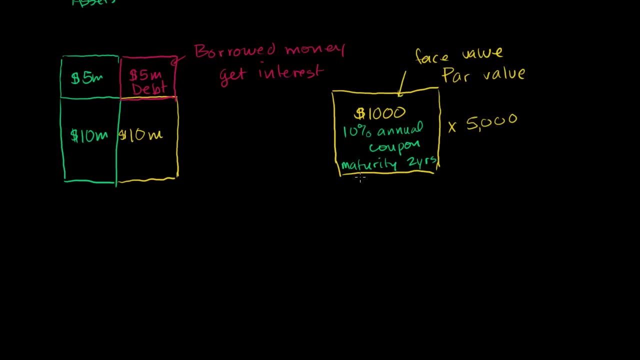 times amongst a bunch of different people, this company would be able to raise its $5 million. Now, just to be clear how the actual payments work: the coupons tend to get paid semi-annually, So let me draw a little timeline. Let me draw a little timeline here. 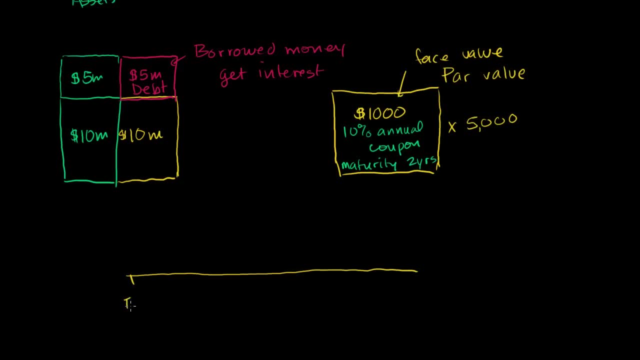 And this tends to be the case in the US and Western Europe. If this is today, this is today, this is in six months, this is in 12 months or one year, this is in 18 months and this is in 24 months. 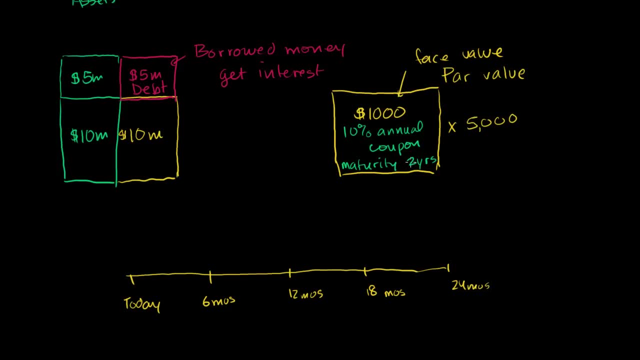 And I'm only going up to 24 months because I said this bond matures in 24 months. So what is this? If you own, if you hold this bond, this certificate, what do you get? Well, it's going to pay you 10% annually. 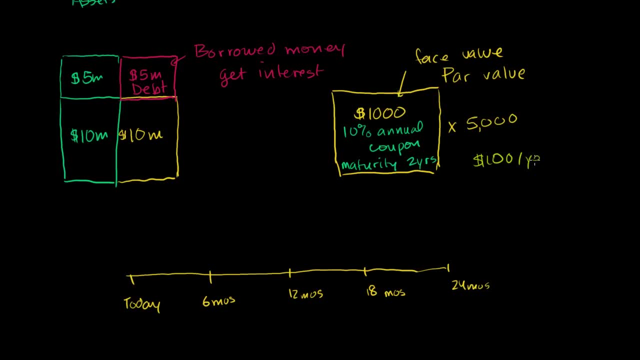 So $100 a year, But they actually pay the coupon semi-annually. So you get $100 a year but you get half of it every six months. So you're going to get $50 after six months. you're going to get $50 after 12 months or after another six months. 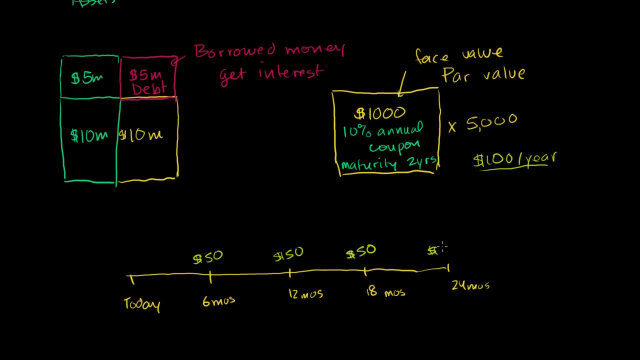 you're going to get another $50 here, you're going to get a final $50 there and they're also going to have to pay you back the original amount of the loan. They're also going to have to pay you a the $1,000.